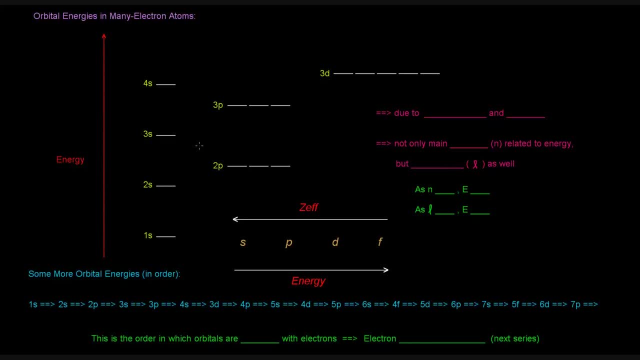 The 2p orbital. The 2p orbital is higher than that in energy. Then there's the 3s orbital, Then there's the 3p orbital, Then there's the 4s orbital, And then there's the 3d orbital. that's a little bit higher in energy than the 4s orbital. 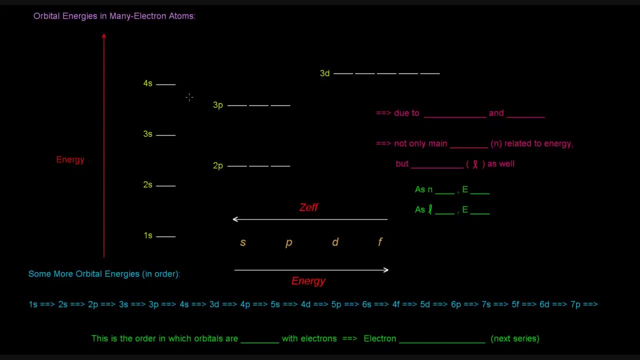 So what's going on here? The idea here, though, is that it's not just the principal quantum number that's important in terms of determining the energy level of that orbital Okay, Because otherwise you would see The case where you saw in the hydrogen atom, where, if you have the same principal quantum number, you have the same energy level. 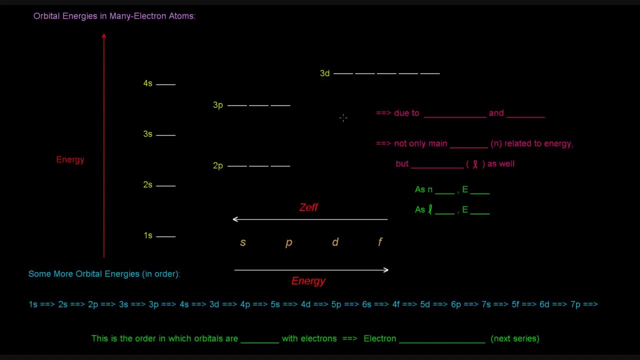 That's not the case. So what's the reason for this? The reason for this is this is due to shielding and effective nuclear charge, And so basically, what happens here is that not only is the main shell right, the principal quantum number or n value, excuse me, related to energy, but the sub-shell. 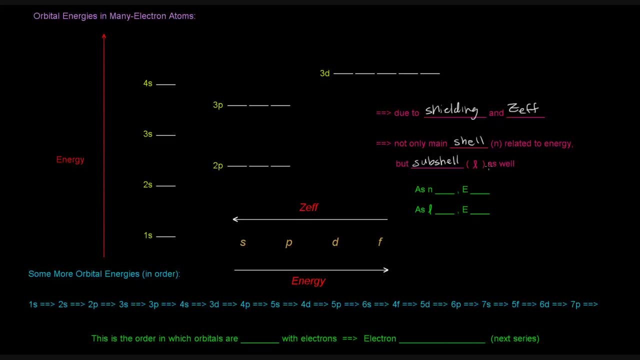 Is related to energy as well. Okay, So we already know that as n increases, the energy of the orbital increases, But in addition to that, as the l value increases, the energy increases as well. Right, We see that here. And that's again due to the effective nuclear charge that we mentioned in the previous video, right, 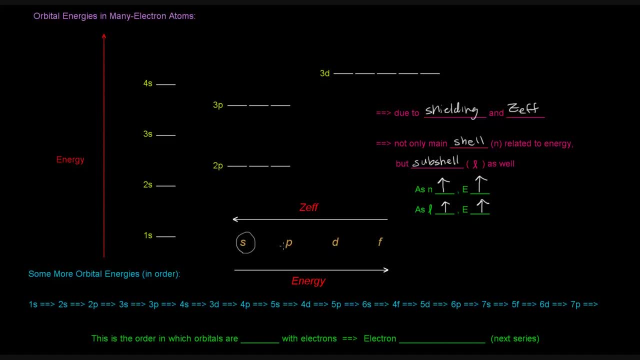 The s orbitals have lower energy than the p, which have lower energy than the d and lower energy than the f. So the f orbitals are the highest in energy And that's because of the effective nuclear charge differences which we talked about in the previous video. 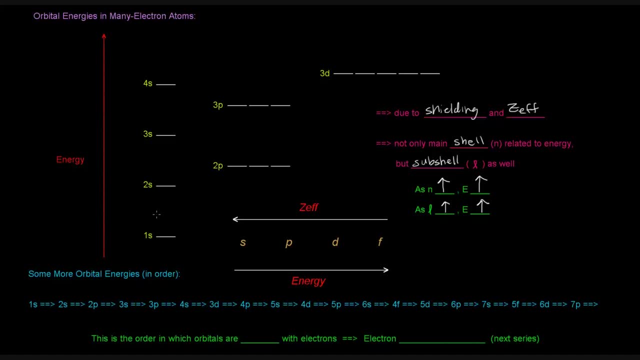 So now you'll notice here that I didn't really put all of the orbitals in this energy diagram, So the others are kind of listed here. So we go from 1s. We already mentioned that we go from 1s to 2s. 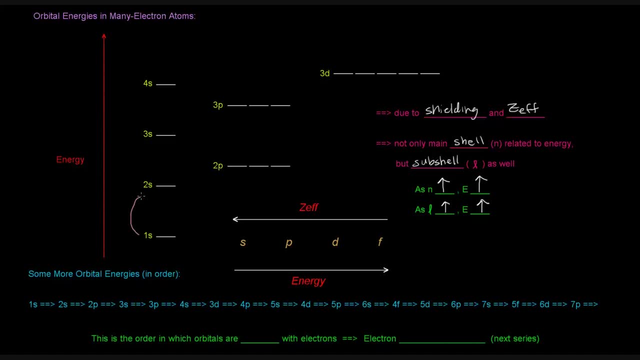 Let's put this in a different color. Let's do this: So: 1s, then it goes to 2s, then there's 2p, then there's 3s, then there's 3p, then there's 4s and then there's 3d.